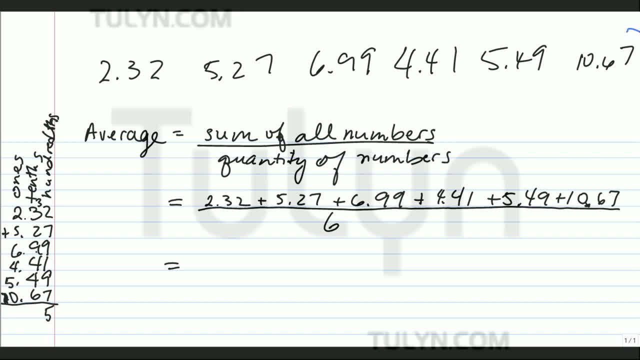 3 plus 3 is 6.. 6 plus 2 is 8.. 8 plus 9 is 17.. 17 plus 4 is 21.. 21 plus 4 is 25.. 25 plus 6 is 31.. 3 plus 2 is 5.. 5 plus 5 is 10.. 10 plus 6 is 16.. 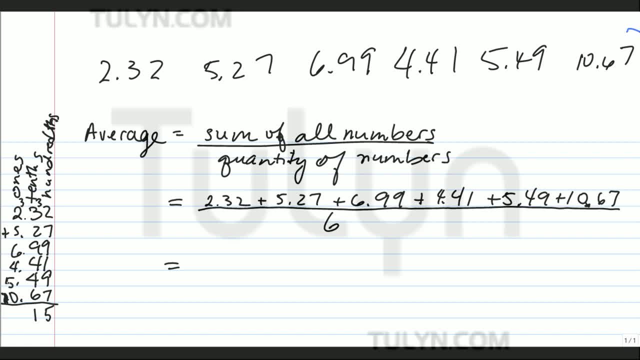 16 plus 4 is 20.. 20 plus 5,, 25.. Carry the 2 up here. 2 plus 1 is 3.. Now make sure see how your decimals are lined up right And that you carry it straight down to center. So I'm going to put your the final answer for. 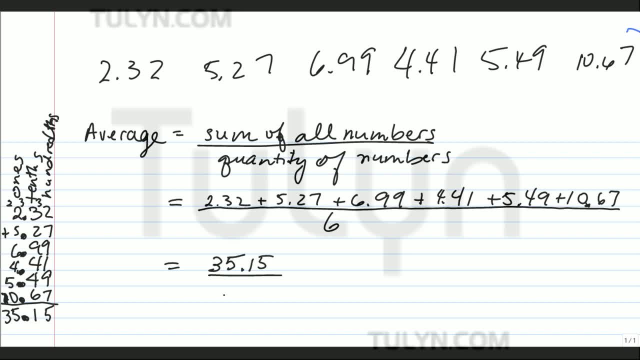 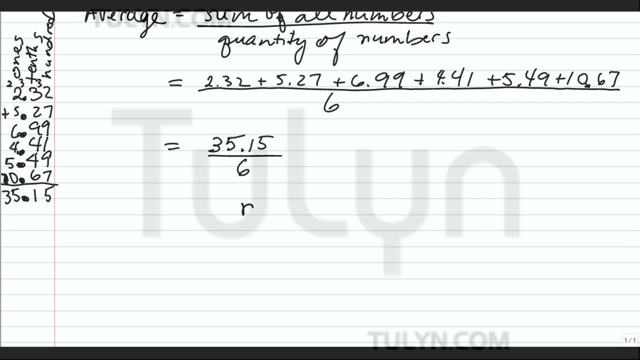 the addition at the top And then replace the division sign, Put back the denominator of 6. And I'm going to divide Now. remember that the formula is like the numerator on the inside and the denominator on the outside. So your numerator is 35.15.. Divide by 8. And then 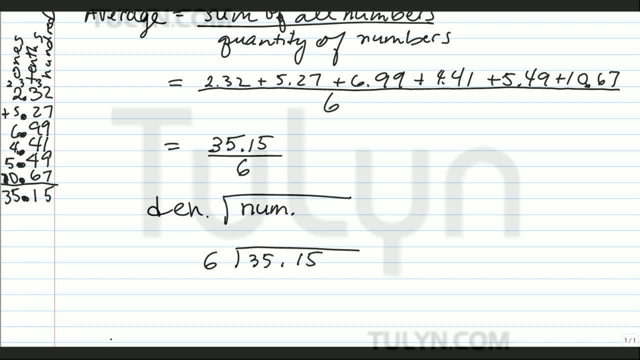 divide by 6.. Now let's look at each number and see if it's divisible by 6.. We've got 3 divided by 6.. Can't do it. 35 divided by 6. Can't do it, It goes in five times Okay. 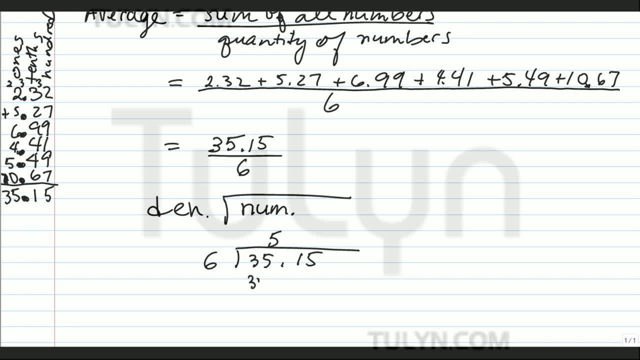 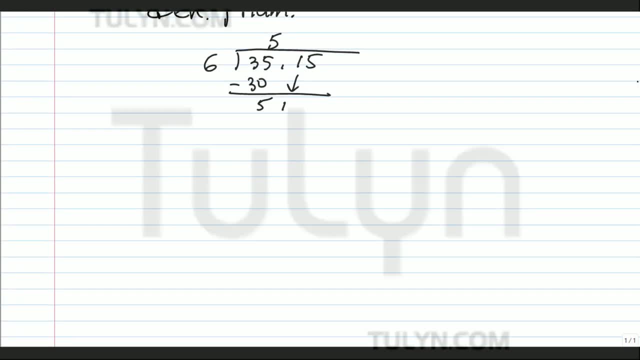 Now you've got: 6 times 5 is 30.. Subtract: 5. Carry down to 1.. 51 divided by 6.. What would that be? 8, correct? Oh, 6 times 8 is 48.. Subtract: 1 minus 8.. Can't do it. And 4 minus 4 is 0., 11 minus. 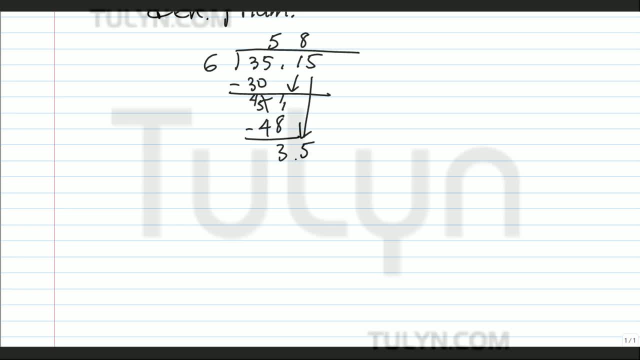 8 is 3.. 35 divided by 6. Goes in five times. That looks a little sloppy. Okay now, 35 divided by 6 is 5.. So 5 times 6 is 30. Subtract by that, 5 minus 8 is 5.. Okay, now go back. 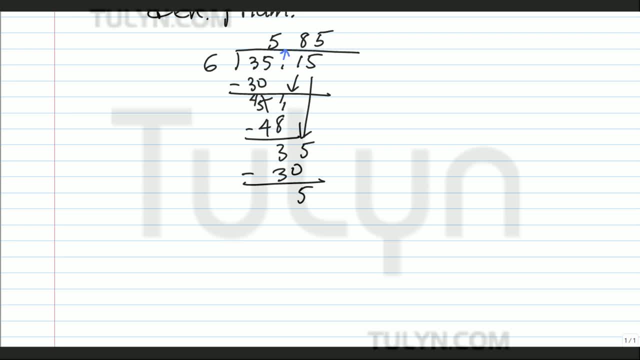 And replace the decimal in your quotient from your dividend to quotient. Okay, now we don't have to round this to the nearest hundredth, because in the back of 5.85 is really an imaginary 0, right And 0 rounds down, So the 5 will remain the same. So the final answer is 5.